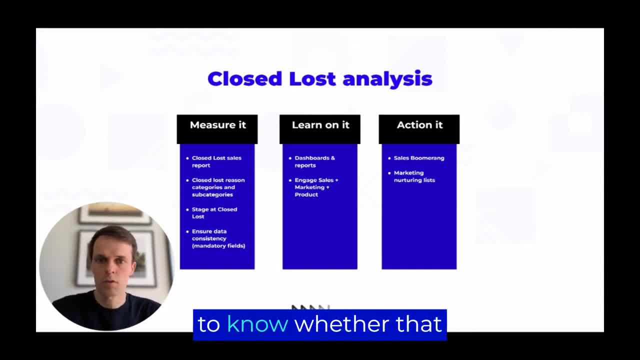 Instead of deciding for a competitor, you would like to know whether that was because of pricing, product fit, payment terms. Of course, collect information on who you are are losing against it, but it's not the loss reason itself. Beside the reason, I recommend capturing the stage. 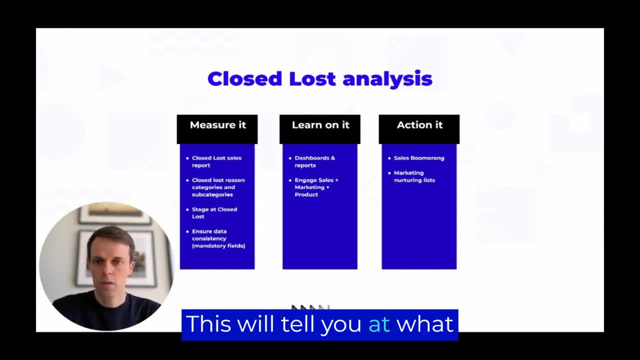 at close lost. This would tell you at what point in the pipeline you have a leaking bucket. You see a high drop after a demo and the primary reason is product too complex for needs. Think how you can showcase the solution differently and focus only on the features that. 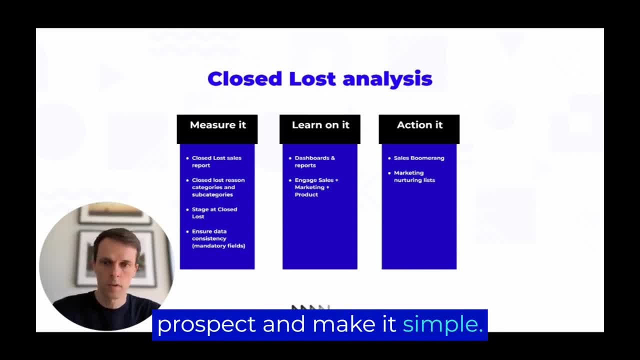 would be relevant for your prospect and make it simple. Lastly, ensure data consistency. Enable the rules in CRM to collect this information in the monetary fields. All right, once you have it measured, learn on it. That's the second pillar. Create dashboard and reports in CRM that would be used by. 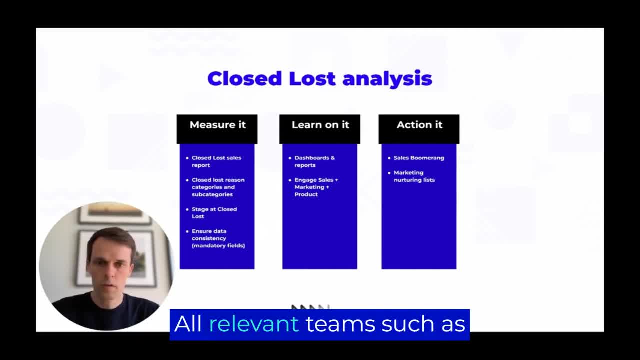 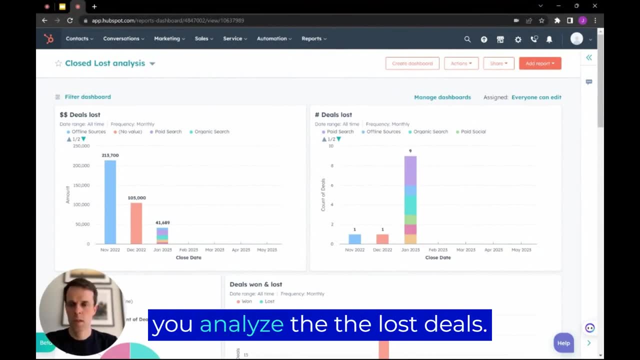 and here is the critical point- all relevant teams, such as sales, obviously, But also marketing and product. Let's see an example dashboard in HubSpot that would help you analyze the lost deals. So, firstly, an overview over time about the volume. 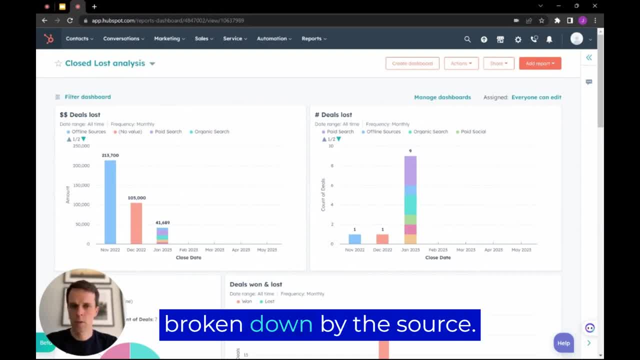 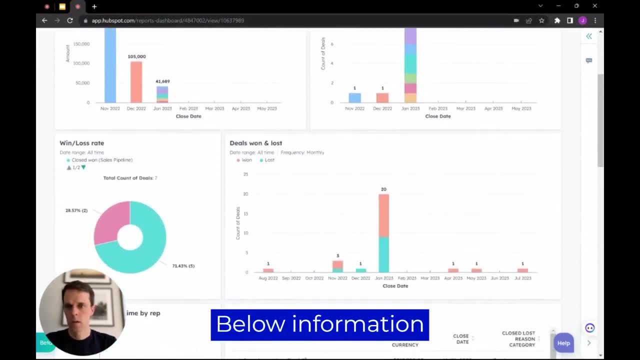 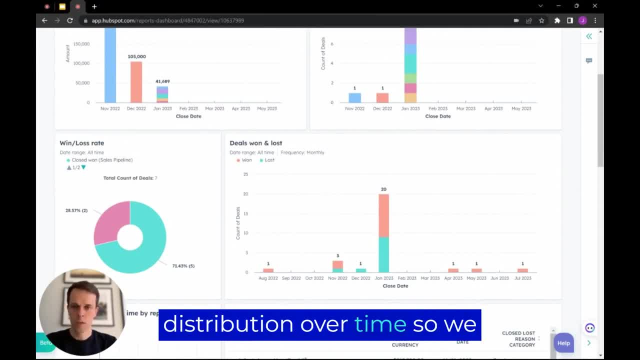 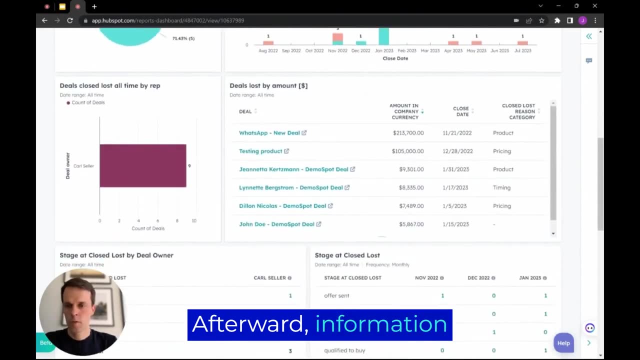 And then the next one, Again with the distribution over time, So we can see the ratio between what you've won and what you've lost And the high-level metric for win and loss rate Afterwards. information about deals lost by rep. 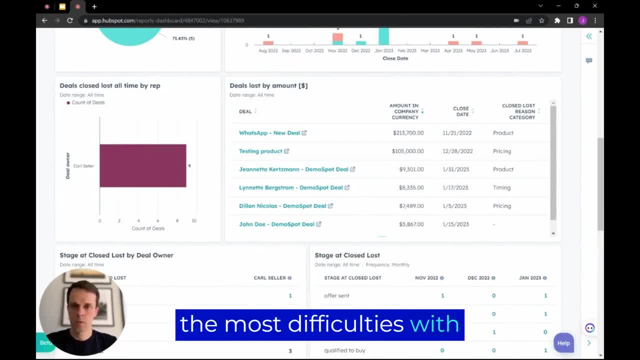 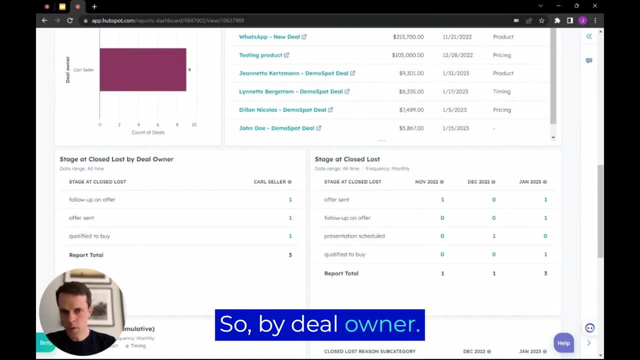 So you can see who is having the most difficulties with closing the deal, as well as the breakdown of individual deals sorted by the amount, Next the stage at close loss, So by deal owner, and distributed over time. So firstly by deal owner, so we can see where specific people have. 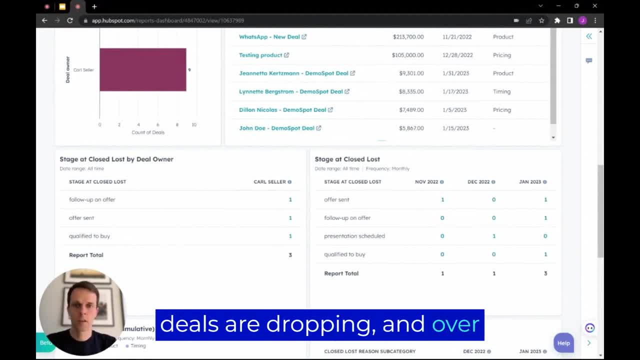 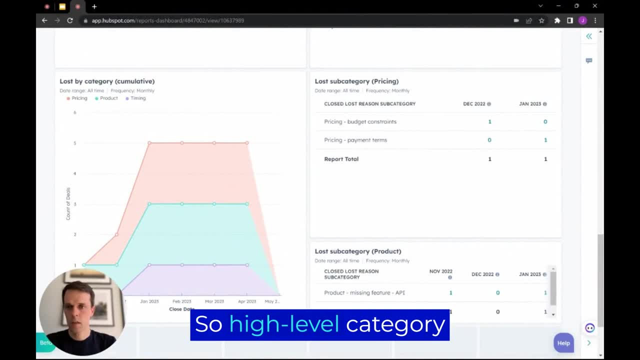 problems and where the deals are dropping And over time, so we can see more trends. And lastly here categories, So high level category, whether it's caused by pricing, whether it's caused by product timing, et cetera. So you can see the cumulative number. 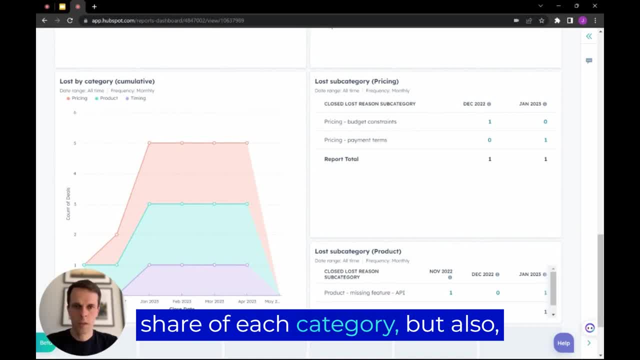 over time and the share of each category, but also breakdown into subcategories. So for pricing, whether it's coming from budget constraints, whether it's coming from payment trends and the likes, product timing and so on, you can replicate depending on the master categories, high level categories that you have for your business. 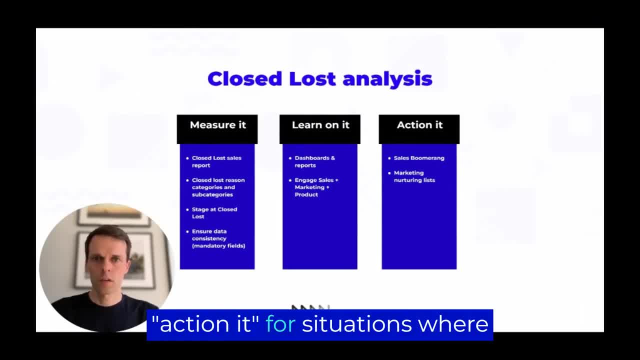 Back to our third pillar, that is, action. it For situations where there is a matter of timing and sales should re-contact prospect in future, have a process in place that would create a task, send a reminder for sales So they re-engage. 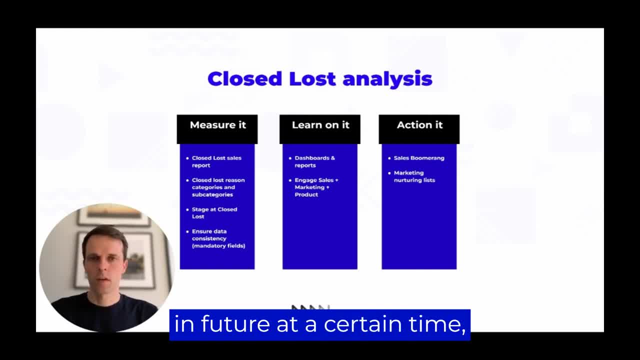 with prospects in future, at a certain time For other cases or on top of that, have nurturing lists and add these deals, add these contacts to these lists, So you create a loop back to marketing to warm up your prospects, For instance, depending on the reasons. 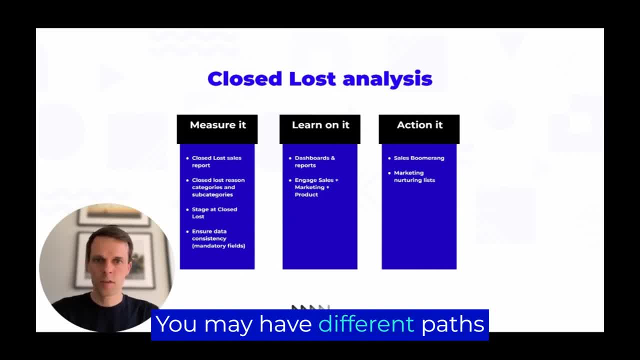 the reason categories that you have. you may have different paths for nurturing. For instance, it's a product to advance or product to complex as a lost reason. send a content marketing to educate and build awareness. So a prospect may not be aware of the critical event or its severity at. 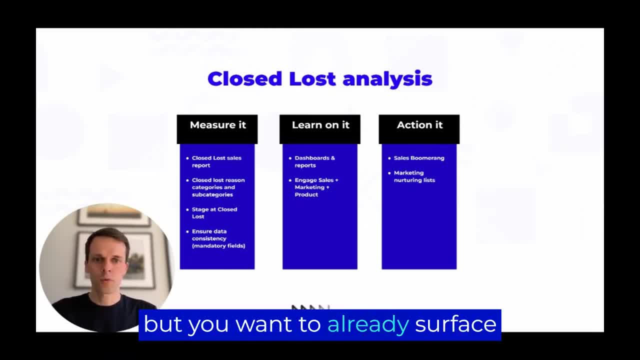 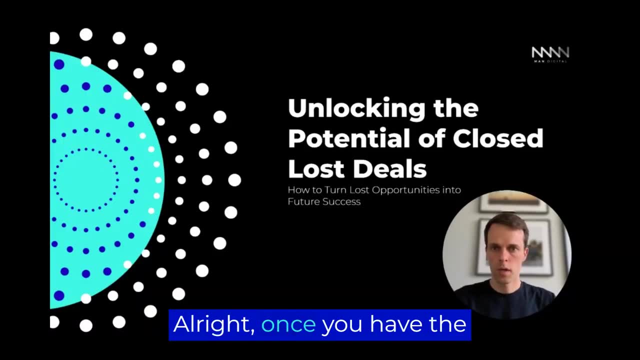 the moment, but you want to already surface the solution, So they have that in mind top of mind. Alternatively for product missing features, send a quarterly newsletter on product updates. All right, once you have the lost analytics implemented, coin that into successful sales.